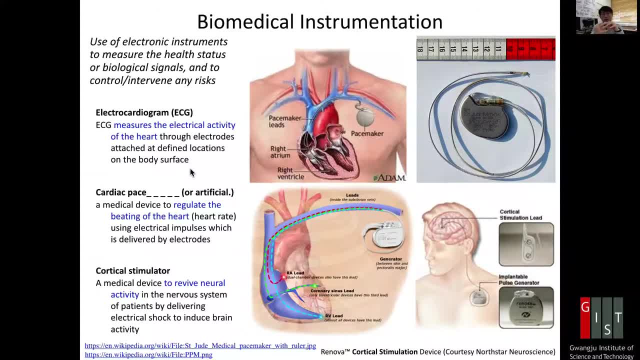 And those patients may have irregular heartbeat which may cause increase of risk And we can have an intervention to externally sending signal to the heart to contract at a regular fashion And that is called pacemaking. So here is called cardiac pacemaker. 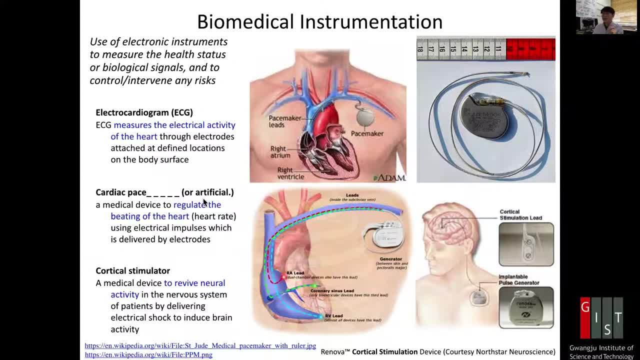 Or we call it artificial pacemaker. This is a medical device to regulate the beating of the heart. Of course, heart rate can be regulated by using sending electrical impulses, which is delivered directly through electrodes inside heart muscle, And another example is called cortical stimulator. 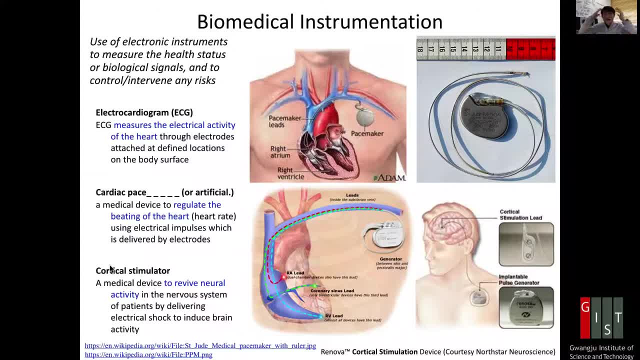 And this cortex means in fact the outer layer of the brain, So cerebral cortex. So this medical device is to revive neural activity in the nervous system of patients by delivering electrical shock to induce brain activity. So let's take a look for this cardiac pacemaker, which is about this small size. 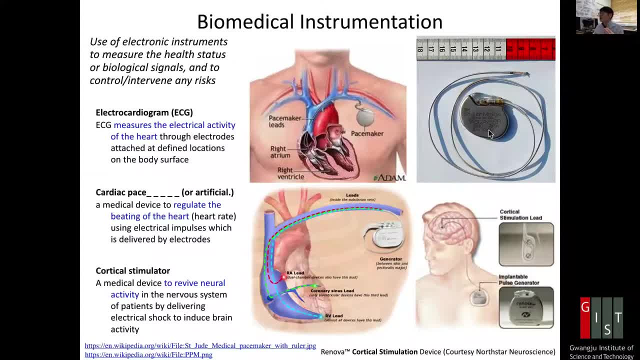 It's not very big And this contains a big plate. It's a battery which sends out electrical impulses through this electrode And if you look at this it's a little bit tiny. But at the tip of the electrode it is a wire which is whoring and neater, so that you actually insert into the heart by rotating and then fix it. 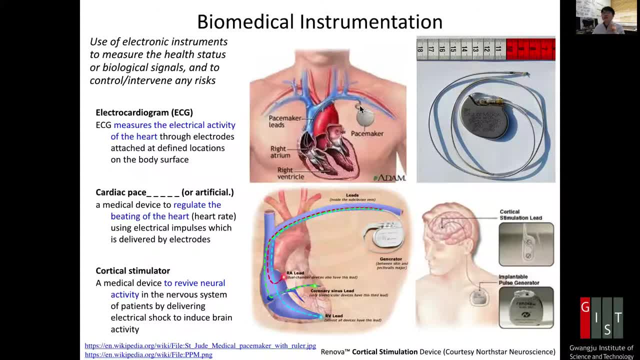 So this pacemaker lead goes through the wall of the vein Which is connected directly to the heart, From your heart anatomy knowledge these veins goes to right atrium And it's right atrium is connected to right ventricle, So it goes to tip of the right ventricle. 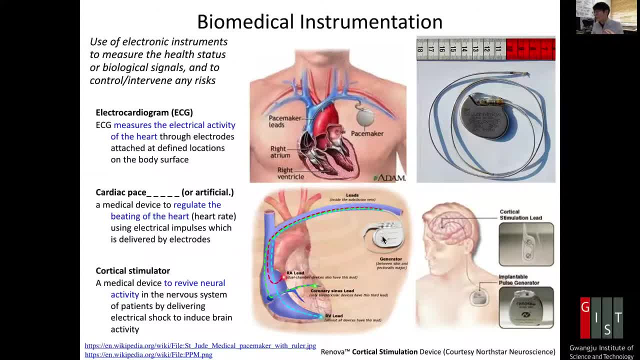 So more specifically, you can see, So this generator is placed surgically inside the body And it goes to subclavian vein, Which is connected to right atrium And you can have right atrial lead or coronary sinus lead or right ventricle lead.